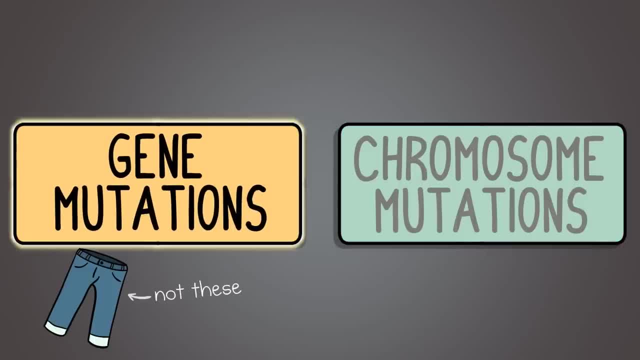 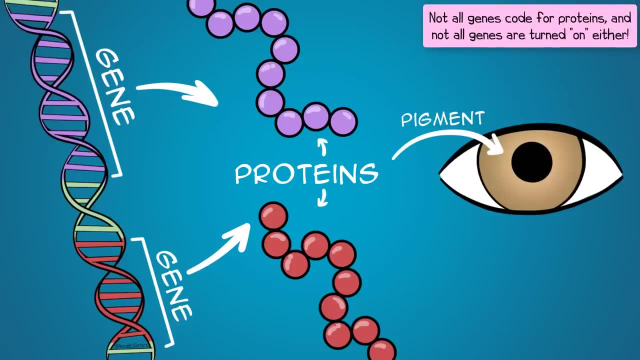 some different types of mutations. We'll start with gene mutations. DNA makes up genes and genes can code for a protein to influence different traits. So when a mutation in DNA happens, which specifically means a change in one or more DNA bases, then different proteins. 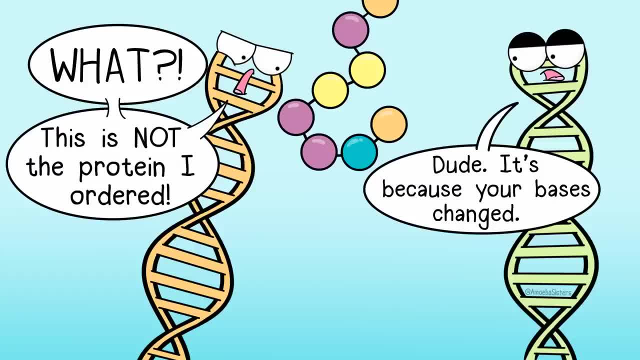 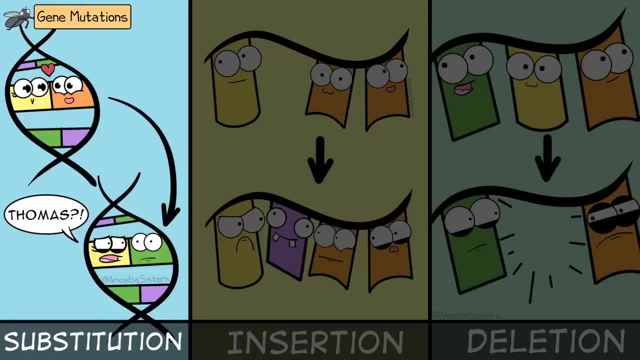 can be produced which can affect an organism's traits. In this example, we have fruit fly. DNA Mutations could include substitution, which means the wrong bases, matched Insertion, which means an extra base, And in this case we have a. 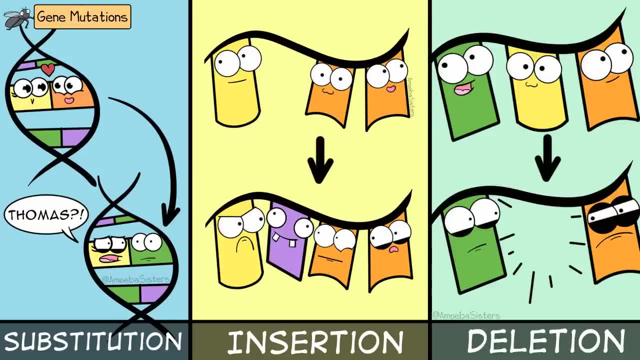 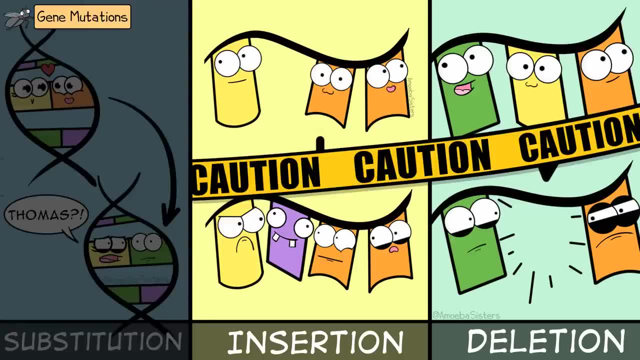 base are added in. There is also deletion, which means a base is removed. Insertions and deletions have the potential to be especially dangerous. Why Remember in protein synthesis how we talked about how bases are read in threes? Well, if you add 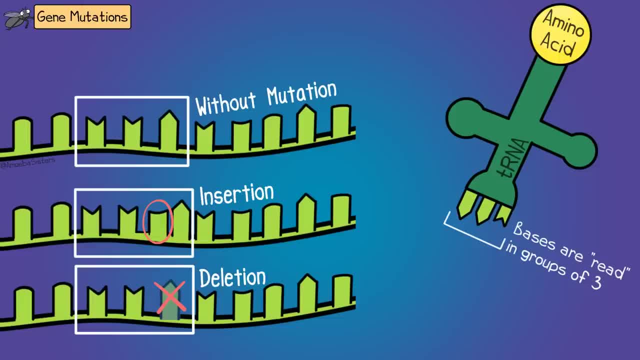 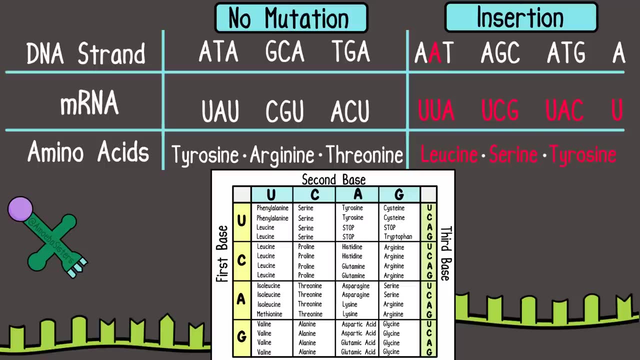 a base or remove a base, suddenly the number of bases total has changed and if you read the bases in threes, depending on where it happened, everything that is read afterwards could be affected. We call this a frameshift mutation. If you look at this frameshift example, 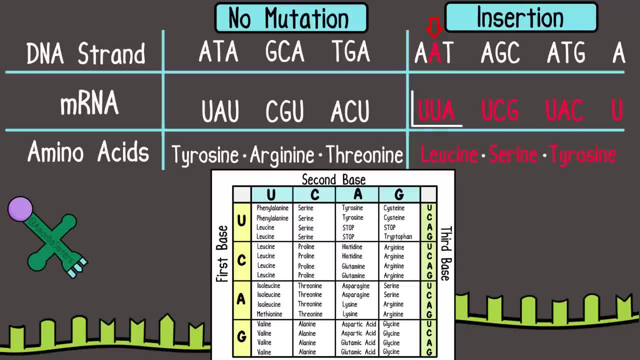 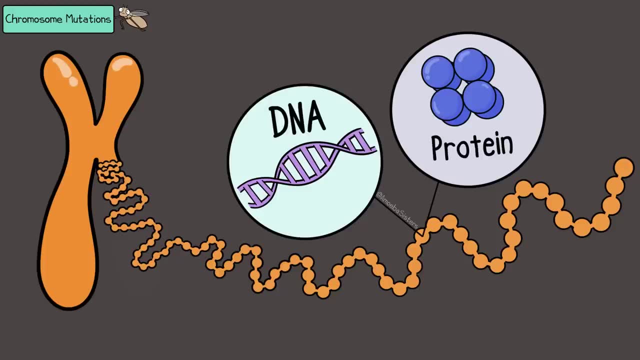 here, where a single base has been inserted, you can see how the following codons, which have three bases each, are now all affected as the reading frame has been shifted. This example shows how it can lead to many amino acid changes. There are also chromosomal mutations. Remember that chromosomes are made up of DNA and protein. 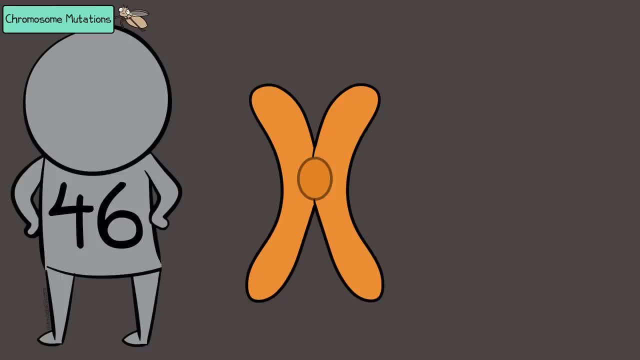 highly organized and they have lots of genes on them. The human chromosome number is the number of genes in the genome. The number of genes in the chromosome number is 46, with 23 from an egg cell and 23 from a sperm cell. This 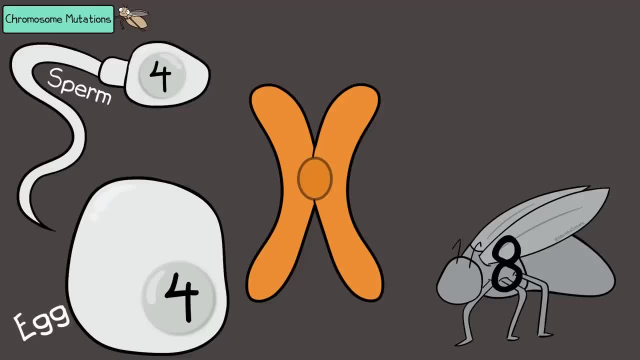 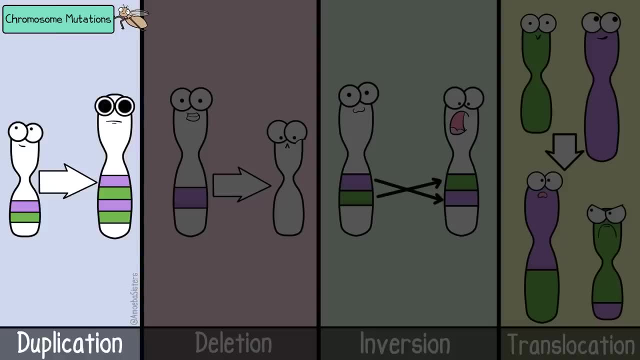 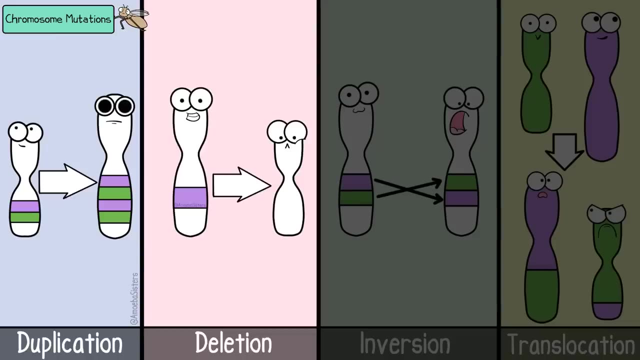 type of fruit fly here, however, has 8 chromosomes, so 4 came from an egg cell and 4 came from a sperm cell. Some examples of chromosomal mutations include duplication, where extra copies of genes are generated. Deletion, where some of the genetic material breaks off. Inversion, when a broken 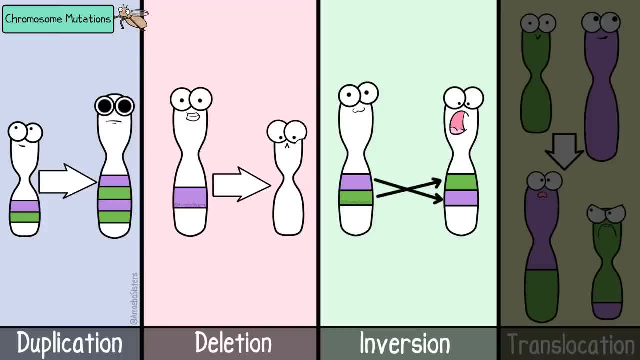 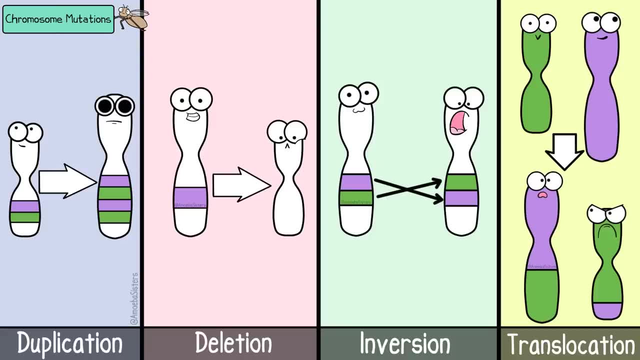 chromosome segment gets inversed, which means reversed and put back on the chromosome, or translocation, when a fragment from one chromosome breaks off and attaches to another chromosome. There's more mutations than what we covered, of course, but the idea is that there are. 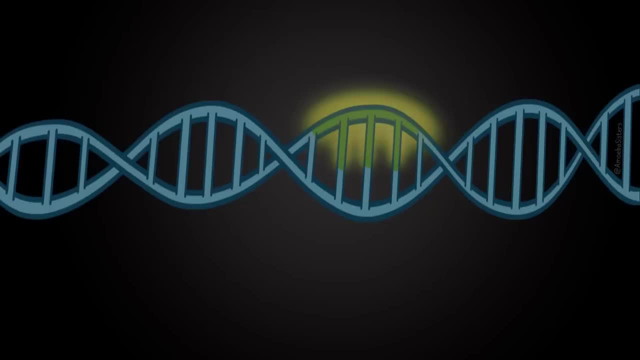 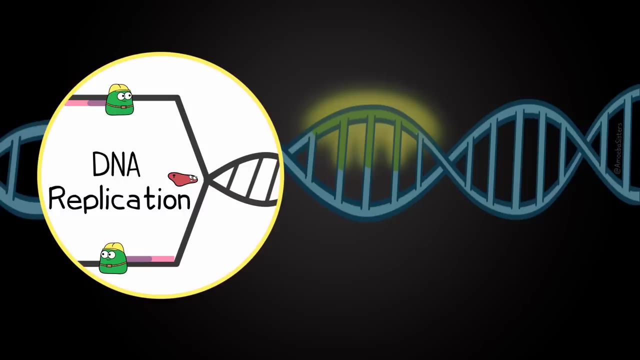 many different kinds of changes that can happen If a mutation is going to happen. we already mentioned that there are especially vulnerable times, such as during DNA replication, But also there are other times too, Like during meiosis In fruit flies and other animals. 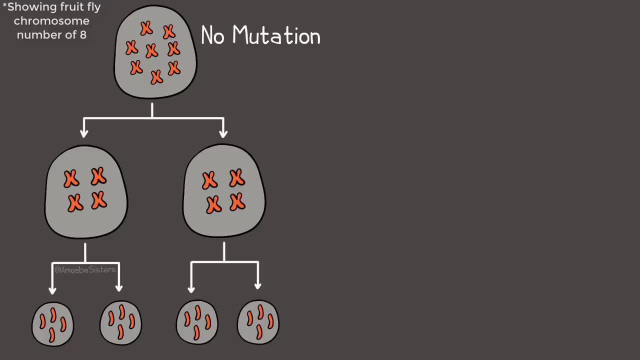 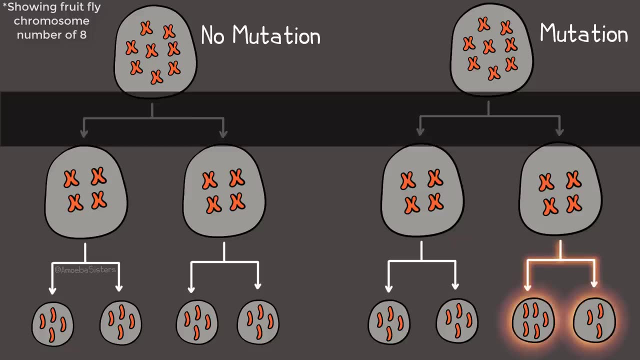 meiosis makes sperm and egg cells. that can happen in the cell. We'll see why that happens. sperm and egg cells that can have half the number of chromosomes as the organism. However, sometimes those chromosomes don't separate completely. We call this nondisjunction. 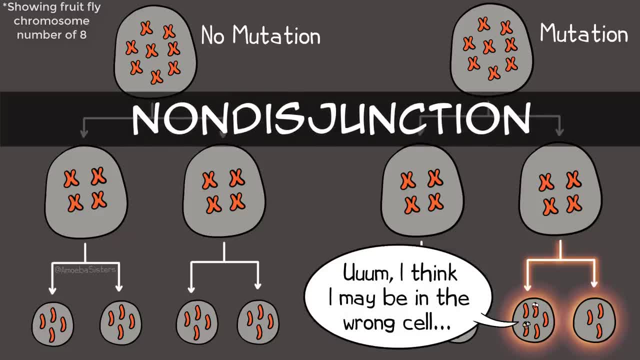 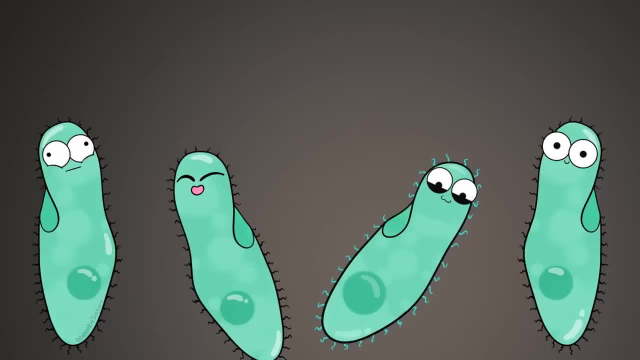 This can result in an egg or sperm cell that has too many or too few chromosomes. It's possible for a mutation to be passed down to offspring. Consider a protist with a mutation. Many protists reproduce asexually, and when they divide, the daughter cell can inherit. 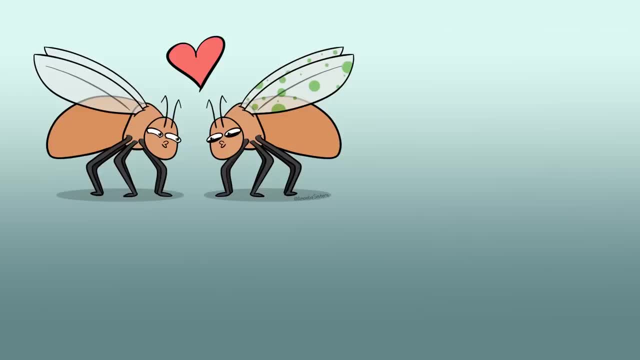 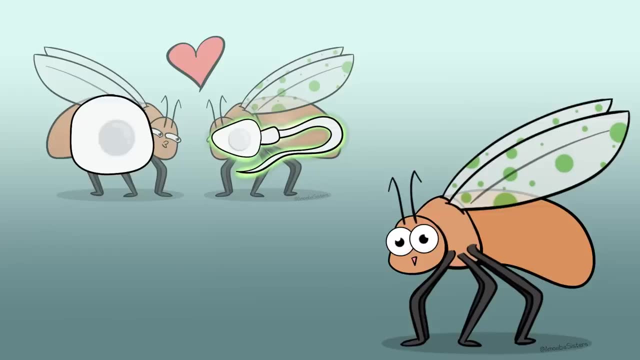 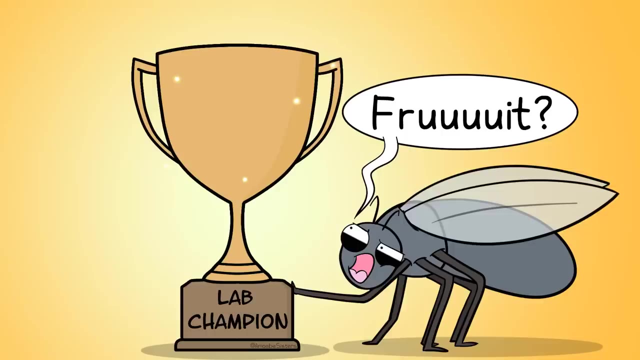 the same mutation. A fruit fly which reproduces sexually can pass a mutation to its offspring if that mutation is found in the genetic material of the sperm or egg cell. You may wonder why we've been mentioning fruit flies so much. Well, they're awesome, but also it turns out that fruit fly mutations and how they 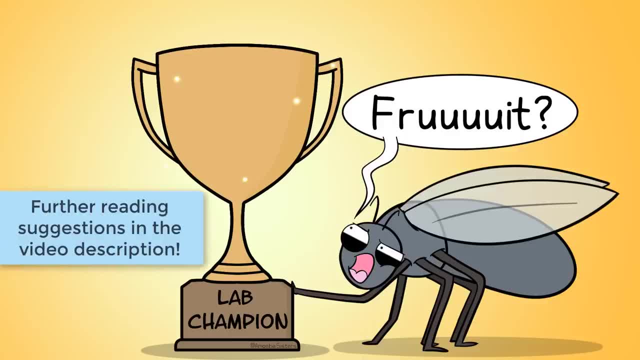 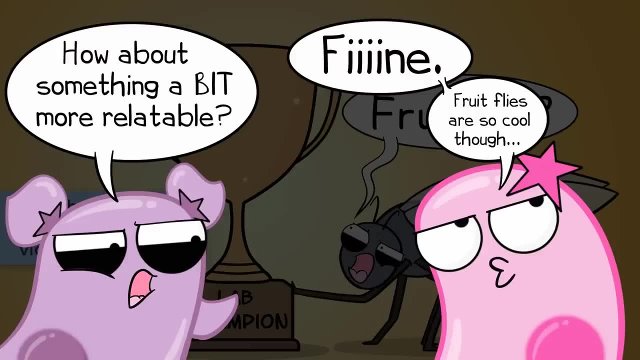 are inherited are frequently studied. We have some links in the video description for more info. These studied mutations can also occur in humans and we'll give a gene mutation example of a substitution in the case of sickle cell anemia. First a little background. 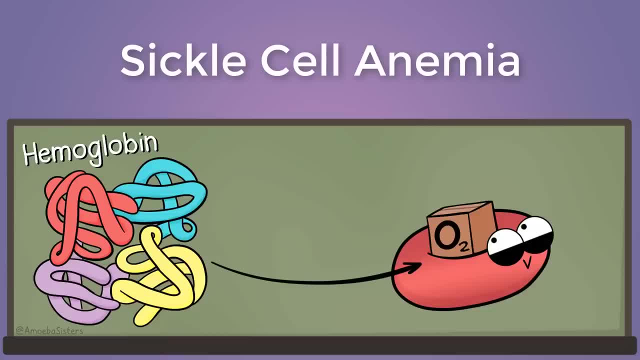 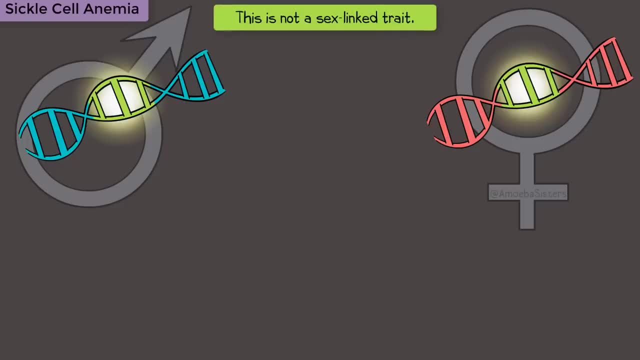 Hemoglobin is a protein in your red blood cells that helps you carry oxygen, But in the disorder sickle cell anemia, the gene that codes for hemoglobin is mutated. If you inherit two copies of this gene, one from each parent, you can have this disorder. 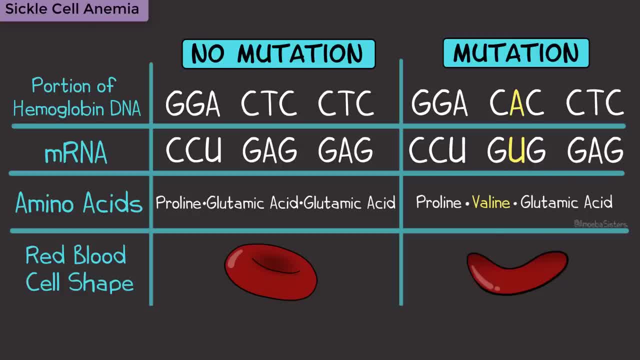 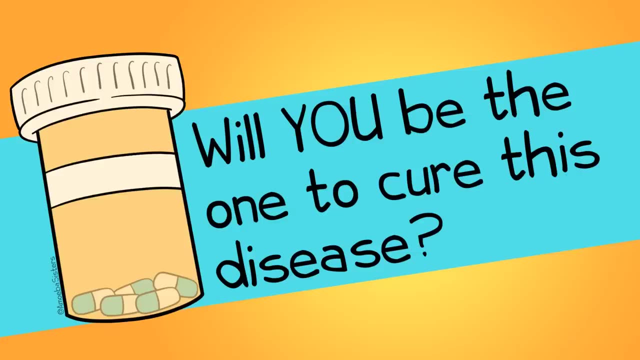 This disorder can make it difficult for your red blood cells to carry oxygen because the shape of the red blood cell is affected from this mutated hemoglobin. This can lead to anemia and other problems. While, unfortunately, there is not a cure for this disorder yet, the good news is that treatment 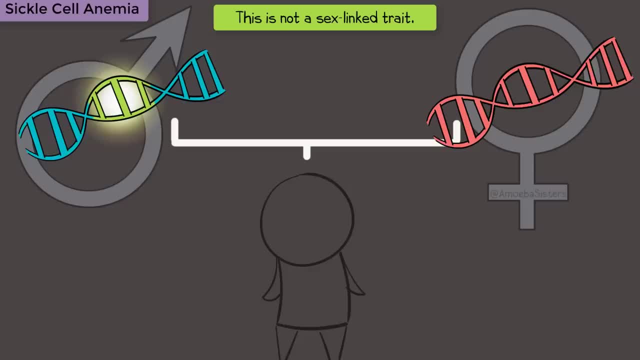 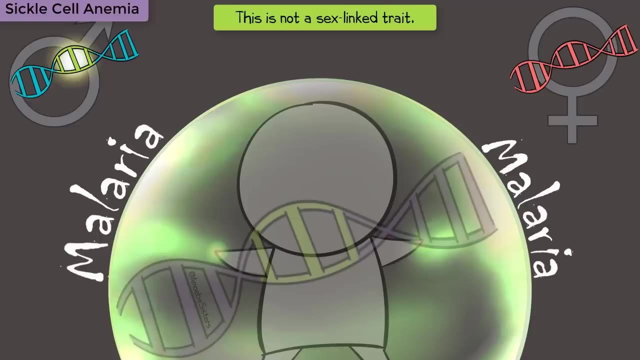 for this disorder has greatly improved. Another thing to mention: if an individual only inherits one copy of the mutated gene from one parent, they are a carrier, but they don't officially have the disease. Usually they do not have symptoms, but those that are carriers appear to have a protective